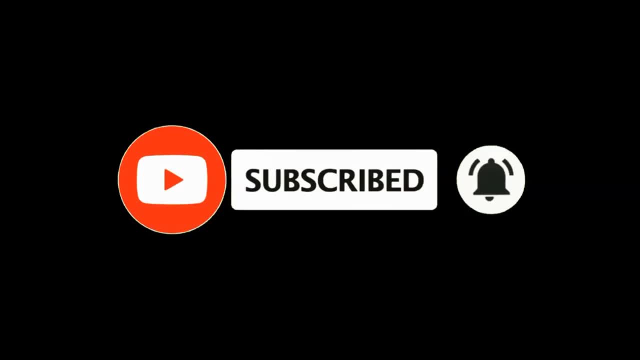 The Geoecologist and please press the bell icon for the updates. Now, sampling is a process of selecting samples from a sample, So we are going to discuss about the sampling techniques and what are the advantages and disadvantages of sampling techniques. So today we are going to discuss 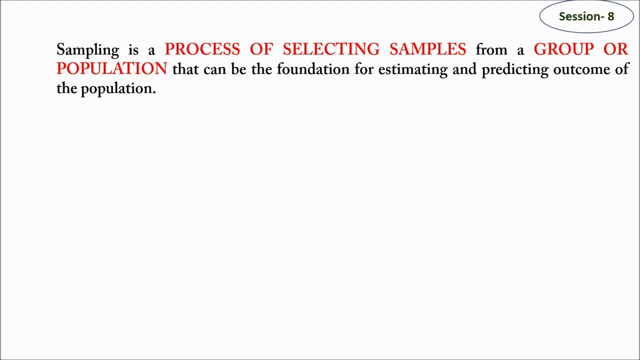 about the sampling techniques and what are the advantages and disadvantages of sampling techniques. So what happens? that it can be the measure of prediction of the outcome that we are looking forward to. So what happens? we sample because we need a smaller group or a population on which 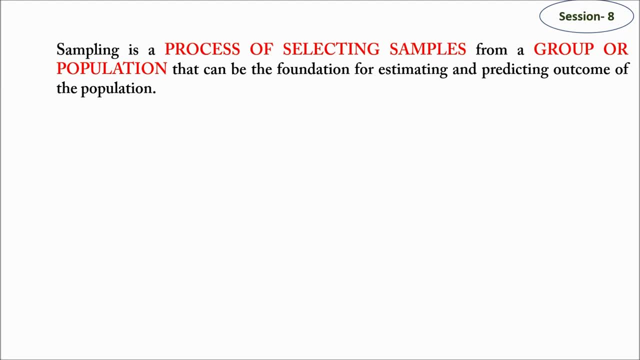 we can predict or estimate the outcome of the entire population. So sampling becomes important. So what happens is that we need a smaller group or a population on which we can predict or estimate the outcome of the entire population. So sampling becomes important for the process of research. It is process of selecting samples from a group or population that we call 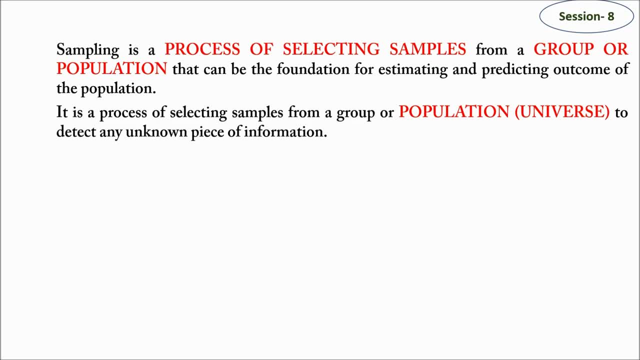 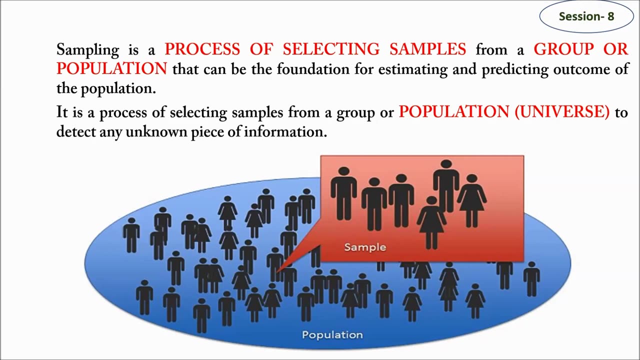 universe. So remember, universe is the total, it's the completeness of the population from which we select the samples. Alright, So in this image, if you see the entire population and only the sample from the population that we select, So the entire population is universe and the part that we select. 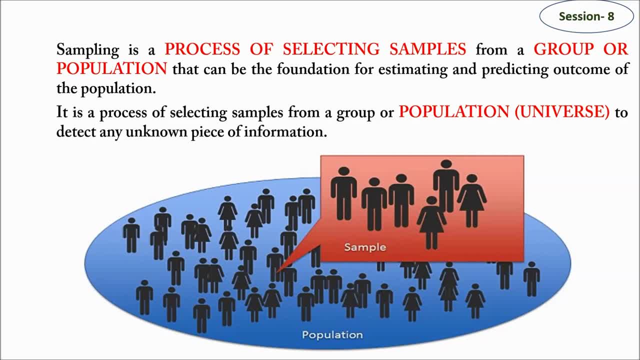 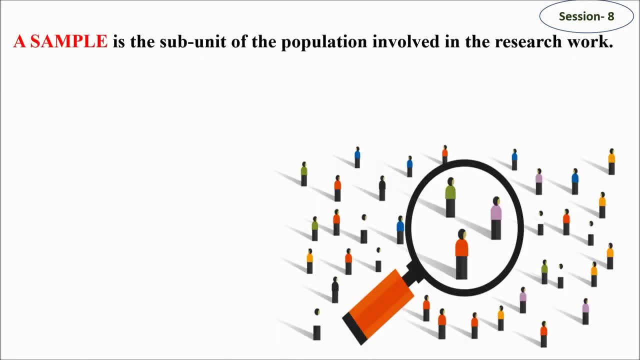 for our study, for estimation, for prediction, for analysis. that part is called Sample. all right, Now let's go further and look. A sample is the sub unit of the population involved in research work. The population is defined by the researcher himself. 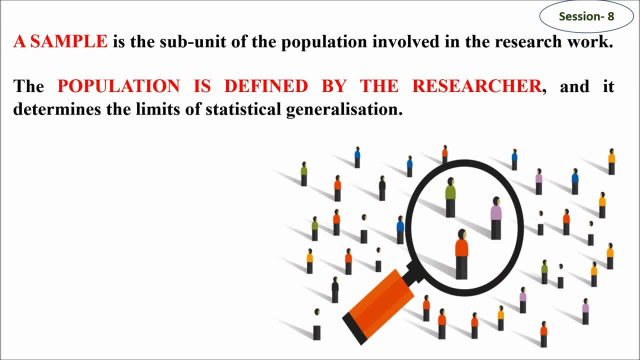 So researcher has to define the population and also the limits of statistical generalization with it. Alright. so often in Geographical research one may not actually want to observe, observe each and every unit in a population. so what happens? sampling becomes most important aspect of geographical inquiry, because a geographer or a social scientist need not. 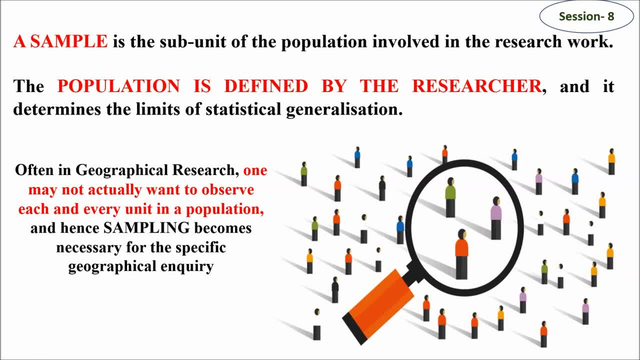 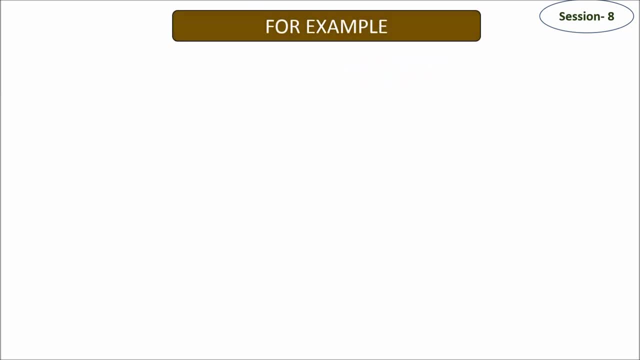 necessarily go to every person, in the entire sample, in the entire population. so sample becomes one of the most handy tool for any geographical inquiry. all right, so, for example, let's look at certain terminologies associated with the sampling process. so let's look at that: a group of elderly. 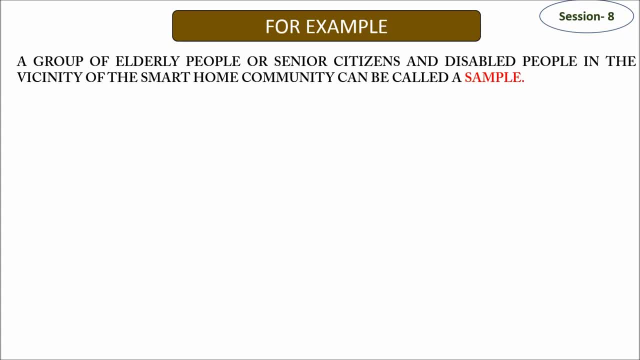 people or senior citizens and disabled people in the vicinity of a smart home community. okay, so suppose there is a situation where we have elderly people or senior citizens or disabled people in a community. so this can be called a sample, because from the population we are selecting only those who are senior citizens or disabled or elderly. okay, so that is a sample. 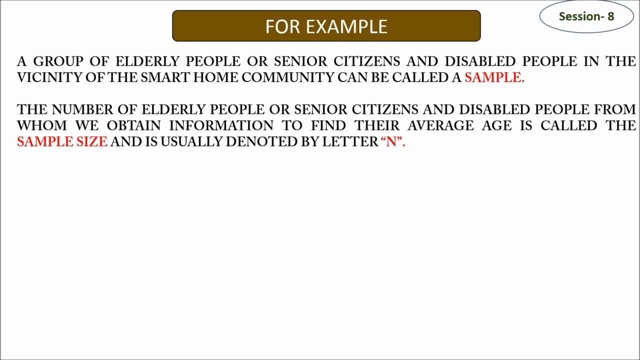 you then what happens? it is referred to n, the capital n or the small n when we talk about the numbers. so that is the sample size that we define. all right. so next is the way we select senior citizens or the sample of disabled people. that is called the design of the sample, or sample design, or 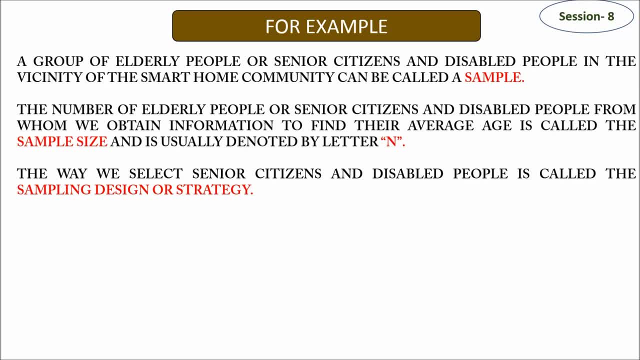 strategy, in what ways we select the sample. that is the sample design or strategy. then each citizen or disabled people that we take out is the important point where selection of our sample is happening. so that is called sampling unit or sampling element. so each unit or each element is important when we 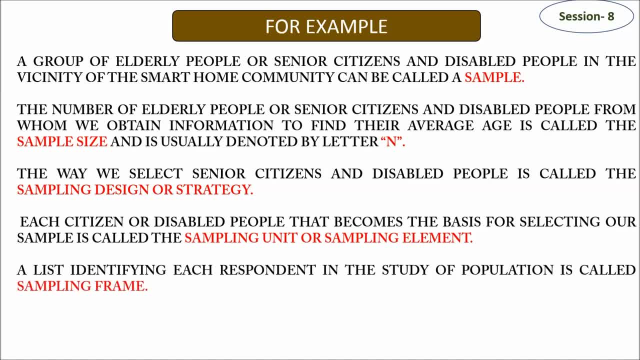 take a sample, all right, the list of identifying each respondent in the study of population. that is called sampling frame. so sampling frame is another terminology. what is it? it's a list that identifies each respondent, okay, in the study of population. and, finally, the obtained results based on the basis of information. 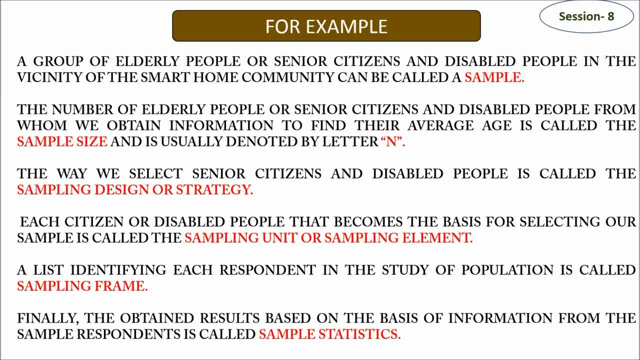 from the sample respondents is called sample statistics. all right, so what did we learn? sample, sample size, sampling design, sampling unit, sampling frame and sampling statistics. so this is the basic idea: taking an example and clearly looking at what a sample means and what are the important terminologies associated with the sample. so now the advantages of sampling can be. 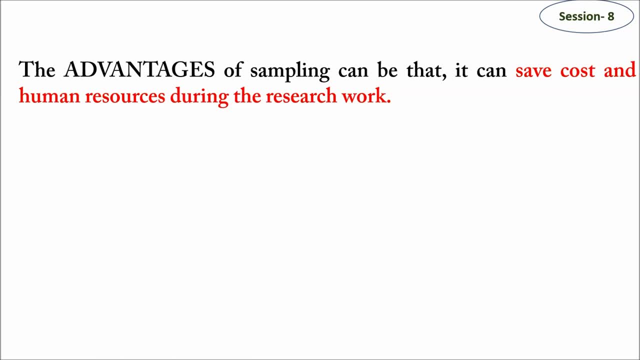 that it saves cost and human resources during research work. all right. and what else this disadvantage can be? a researcher may not find the information about the population being studied specifically to its characteristic and can only estimate or predict them. so, on the basis of sample, the exactness may not be available of the population to be type. so on the basis of sample. the exactness may not be available of the population. notification may not be available of the population to. it is not a whole model and Doctor may not be available of the population because of�� um. if you do um score factor regardless of the actual population. so there might be more red dotdessusES, the % of the population. checking ox quickly. sp Denis only estimate or predict a study topic, so on the basis of sample, the exactness may not be available. on the basis of sample, the exactness may not be available. 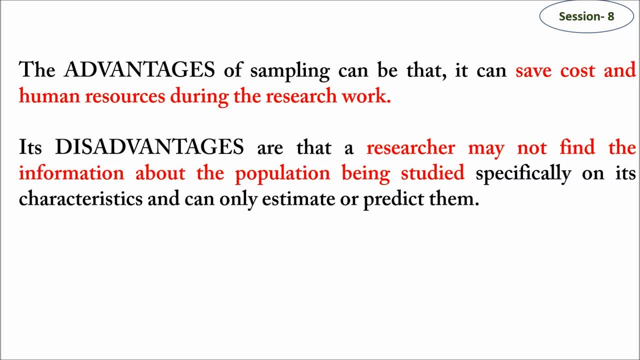 of the population that we are looking forward to as a researcher. so these are the advantages and disadvantage. this means that there is a high possibility of error occurrence. okay, remember this: that using a sample method, an error occurrence has a high probability because it is not linked to. 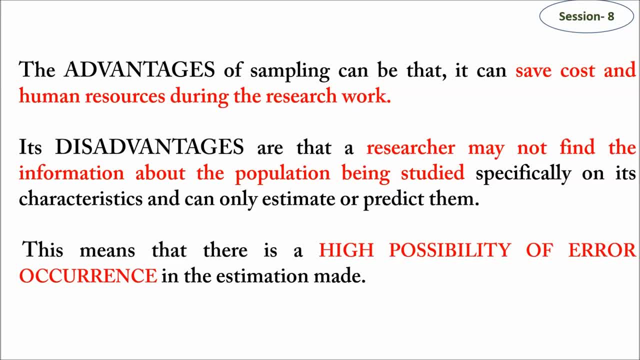 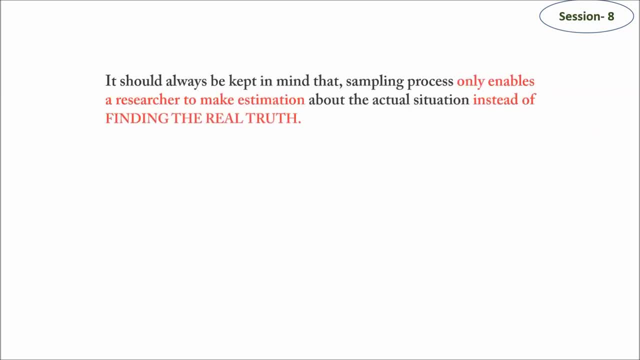 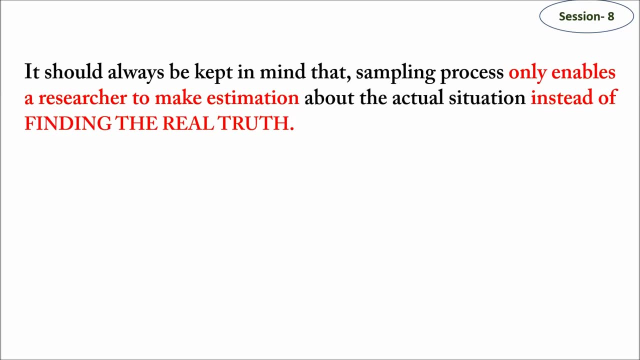 the entire population. it is just holding on to a particular sample size of population. all right, that is much important now. so it should always be kept in mind that sampling process only enables a researcher to make estimation- okay, about the actual situation. so remember, an estimation about the actual situation may not be the real truth, it may be close or away from the real truth. so what? 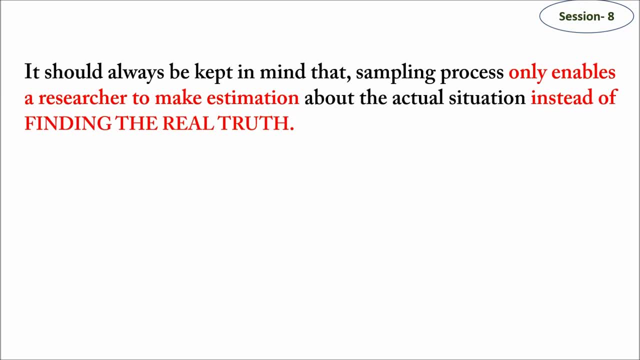 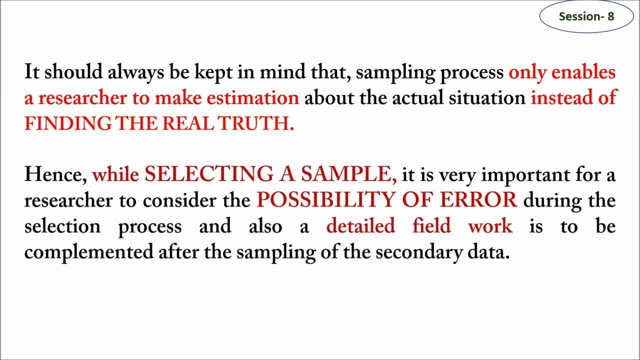 are we doing? using sampling? we are trying to estimate, but the estimation may be, or may not be, close to the real truth. that's why, while selecting a sample, we should be very careful, because there is a possibility of error and hence a detailed fieldwork along with these secondary data. 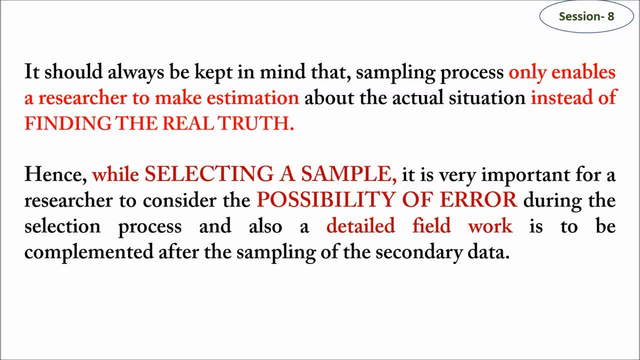 sample is important to complement the research. so if we have a sample taken from a secondary data, we must complement that using the field work and then we can arrive to a better conclusion, a better estimation close to the real truth of the ground. all right, so remember whenever we are taking a sample: 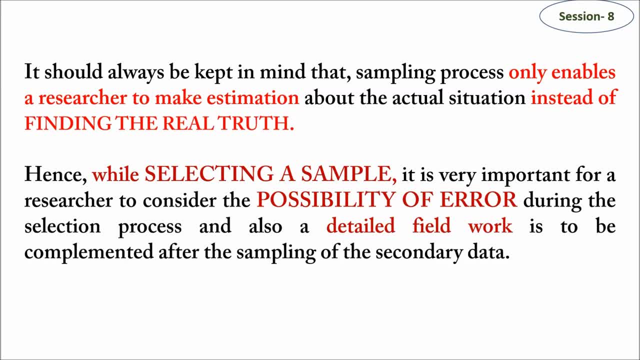 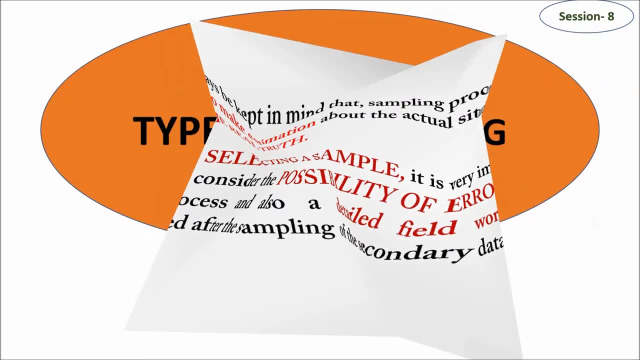 be careful regarding the advantages and disadvantages of the method that we are using. so that we are going to study in the types of sample today. so let's go further. so, types of sampling, all right, so let's go ahead and see what are the major types of sampling. the first is 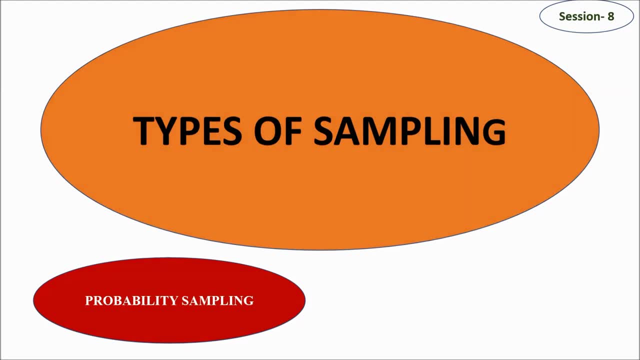 probability sampling and the second is non-probability sampling, as the name suggests. one is based on the probability of estimation, so how probable is the result that we are looking forward to, and the other is non-probability, so it's not based on the chances of occurrence. 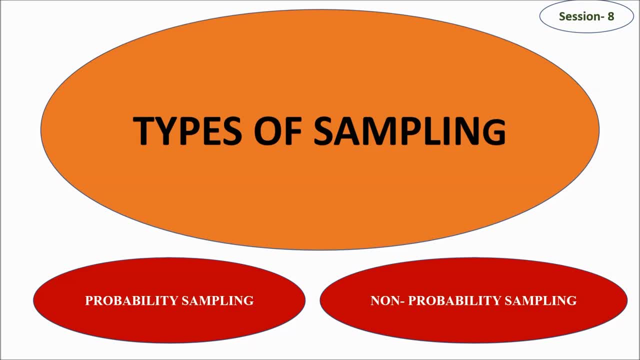 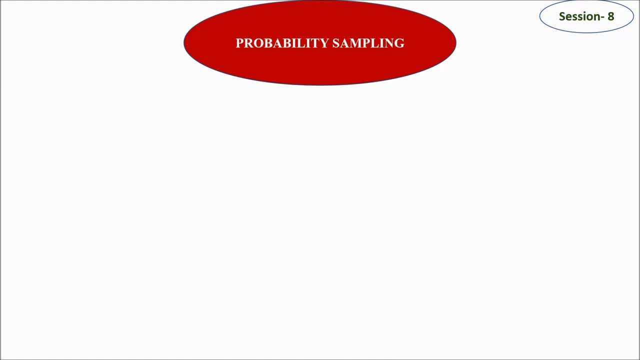 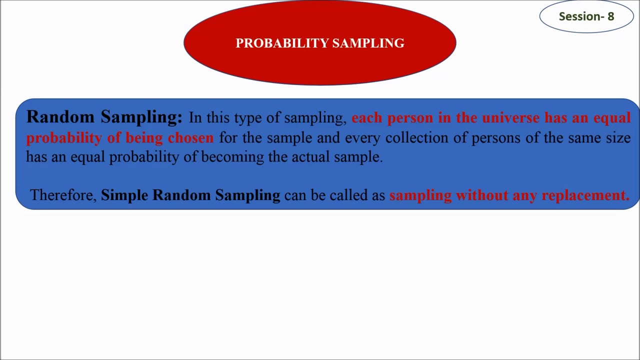 okay, so there are two major segments of types of sampling. now, one by one, we are going to look at each. so first the probability sampling. all right, so first in probability sampling is the random sampling. the word is random, so randomly a sample is selected. it means each person in the universe has an equal probability of being chosen as a sample. so if 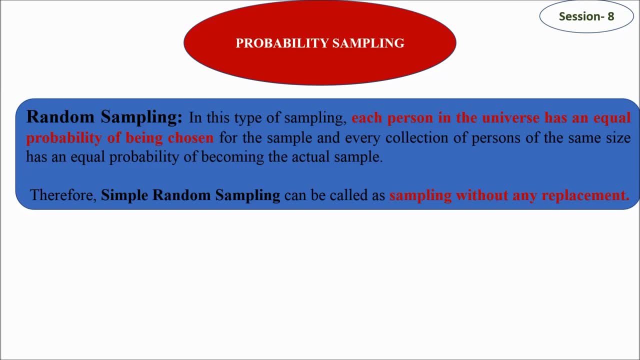 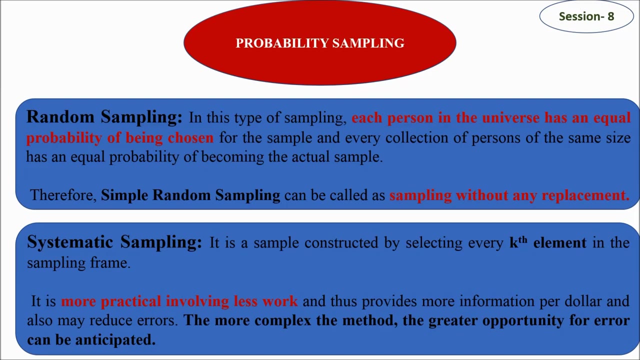 we are choosing. randomly means probability is equal for the entire population or the entire universe from which we select the sample. all right, so simple random sampling can be called also as sampling without any replacement. that is the important point to remember. then we have systematic sampling, so earlier it was a random sampling, then we have systematic sampling. the word itself is systematic. 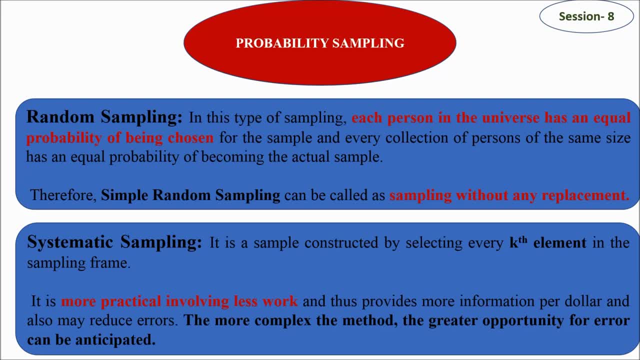 in a systematic manner, for example, kth element, so every kth element that we are selecting in the sample frame, all right. so it is more practical, involving less work, and many times it is complex method, so the greater opportunity for error is also there. all right. so remember, while systematic, 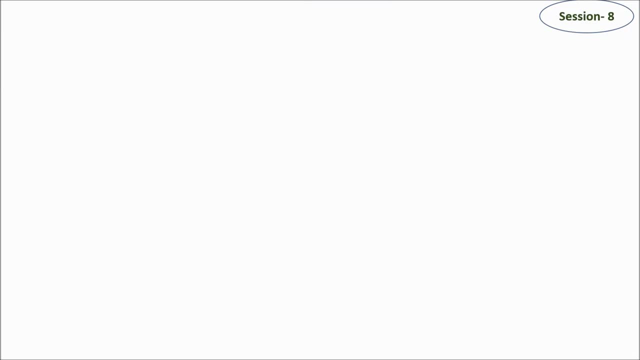 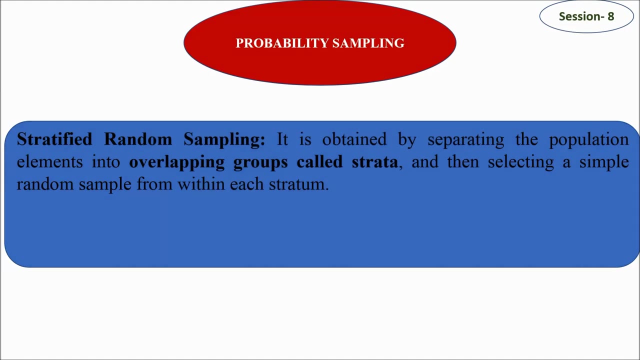 sampling. okay, then what we have is the stratified random sampling. earlier it was just simple: random, now it is stratified random. it means what happens. it is obtained by separating the population elements into overlapping groups called strata. so if we divide the population into various strata and then 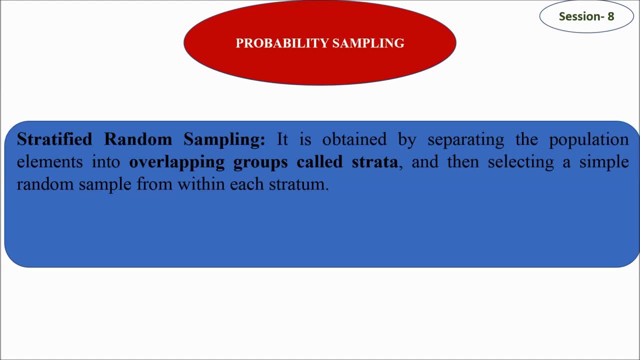 select a simple random sampling from each of the stratum. all right, so this type of sampling is commonly used, very common. stratified random sampling is the most commonly used in geographical research. why? because we have layers of factors, multitude of factors. so what we have, what happens, we divide. 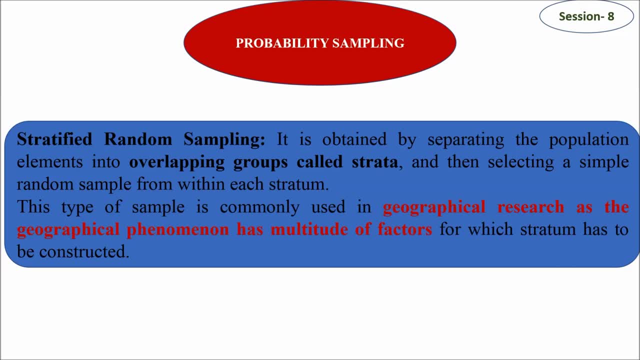 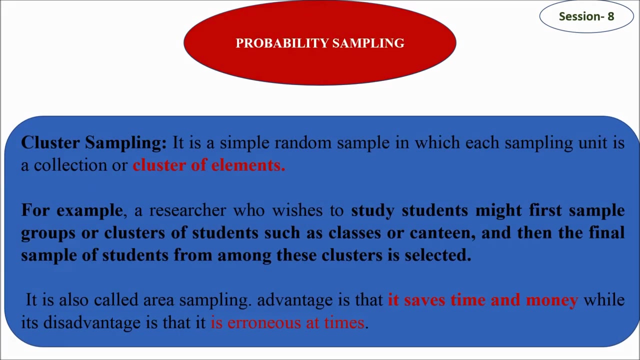 the entire universe, entire population, into those multitude of factors, and then we select the sample from each stratum. all right. that's why stratified random sampling is widely used in geographical research. then what we have is cluster sampling. all right, so, as the term suggests, it's a simple. 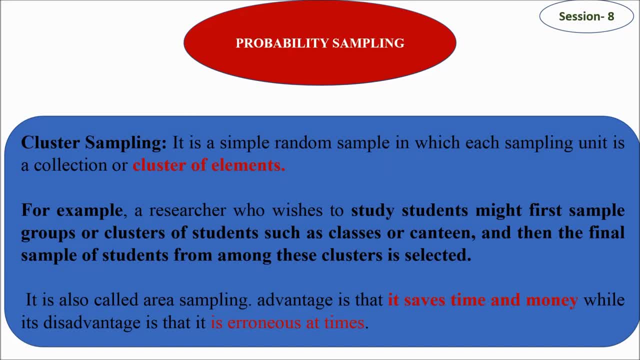 random sample. okay, but it is a unit based on cluster of elements. for example, a researcher who wishes to study students might first sample a group or a cluster of students, such as classes or canteen, and then final sample of students can be selected from these clusters. all right, so it. 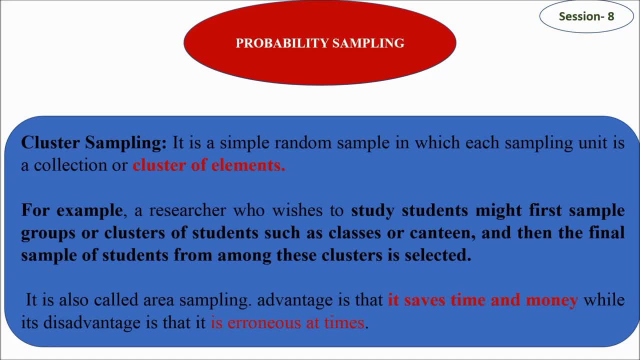 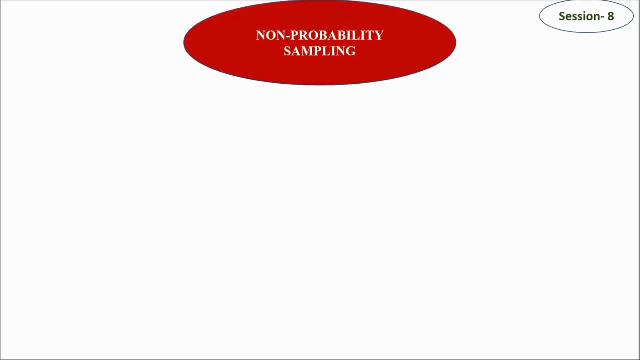 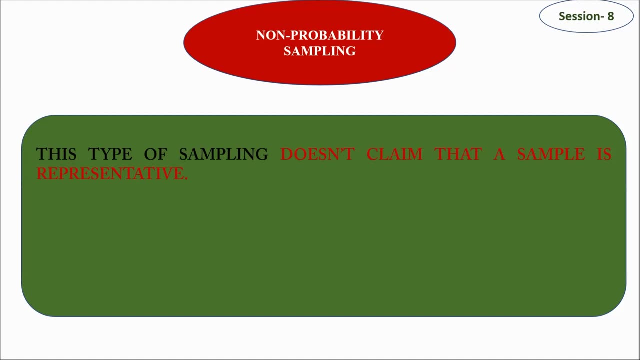 saves time and money, but it can be erroneous as well. all right, so remember, cluster sampling can also have errors in that. all right, then non-probability sampling. so what are the non-probability sampling? the first one: we understand the characteristics. this type of sampling does not claim that a sample is representative probability sample. 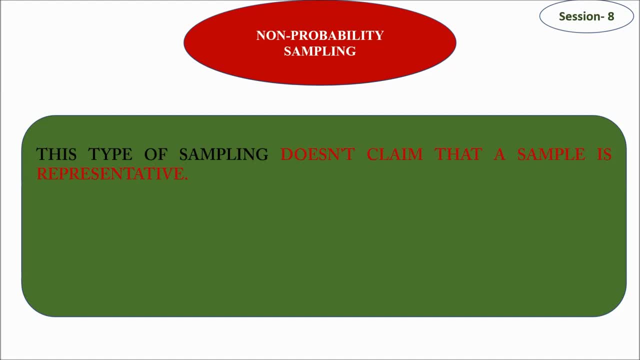 claims that it is representative of the population of the universe, but non-probability sample doesn't claim. it doesn't say that it is the representative of the entire population, all right, so non-probability sampling is less complicated and less expensive as well, so that we need to understand that. 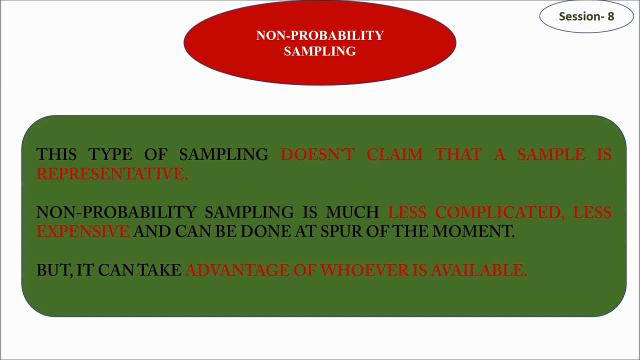 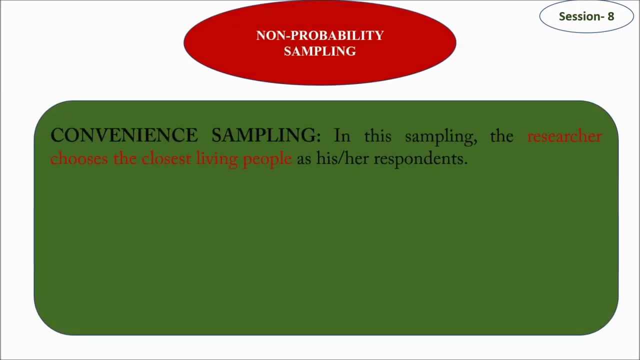 this type of sampling is definitely aassic to remember, but it can be done, you know, taking advantage of whosoever is available as a sample. so the study can be done on the basis of whosoever is available. now let's look at the types. so what is under non probability sample? the first: 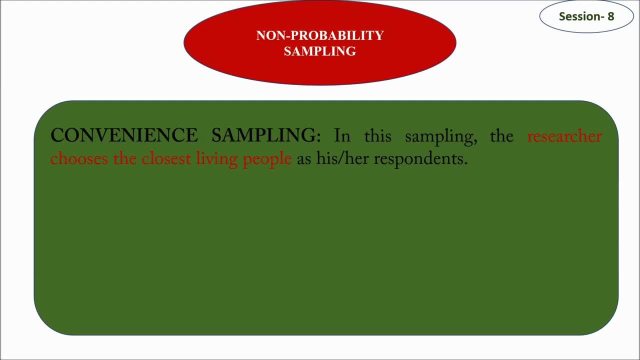 is convenience sampling. the first word itself is convenience, so try and understand. it's about convenience. so the researcher is the person who insights to talk to people about it who are, So respondence is based on the convenience of the researcher. Next is the quota sampling. 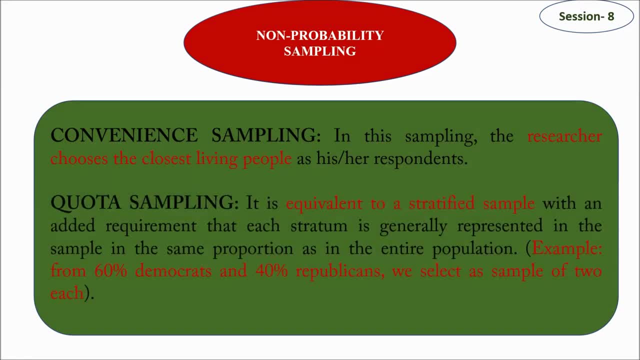 It's very much similar in order to look at it. So it's very similar to stratified sample. So what happens? Quota is being decided, For example, 60% of Democrats and 40% of Republicans as a sample, So this is something like a quota given to a particular group of population, and then 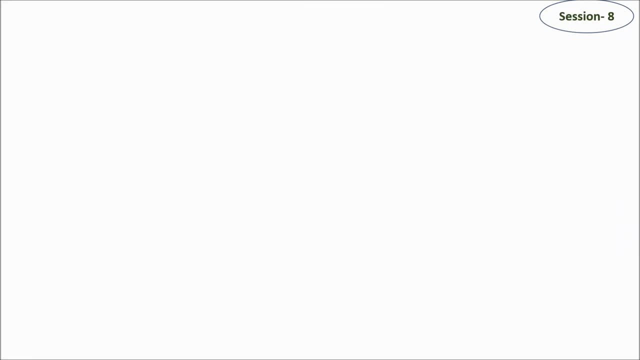 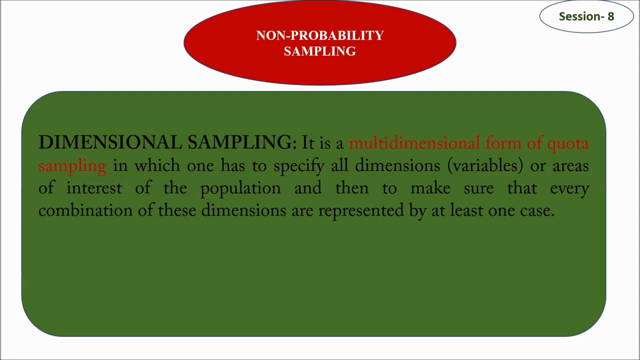 on the basis of that, selecting a sample. Then it's dimensional sampling- very much interesting. It is multi dimensional form of quota sampling in which one has to specify the variables- very much important. and this is very much important in also geographical research, because there are numerous variables. 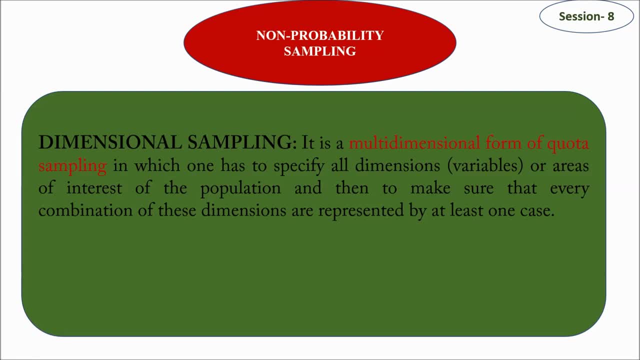 So of interest of population, and then to make sure that every combination of these dimensions are represented at least once, for example soil and slope, soil and vegetation, So similar kind of you know. So relations are there and then multi dimensional form of quota sampling can be done using that. 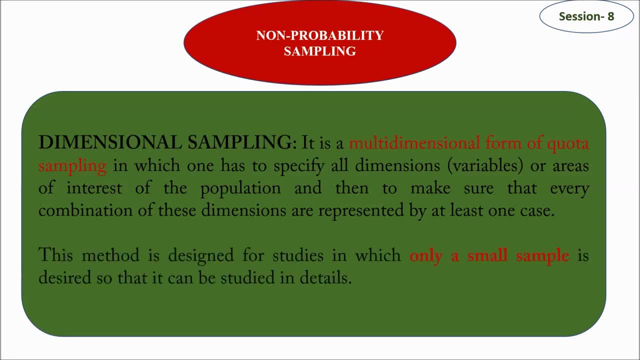 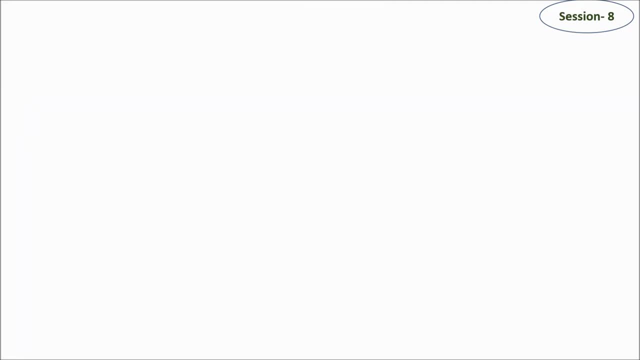 All right. So this method is designed for studies in which only a small sample is required. So in case of small samples, dimensional sampling can be used, then purposive sampling. So purposive is very much to the purpose. So who defines the purpose? 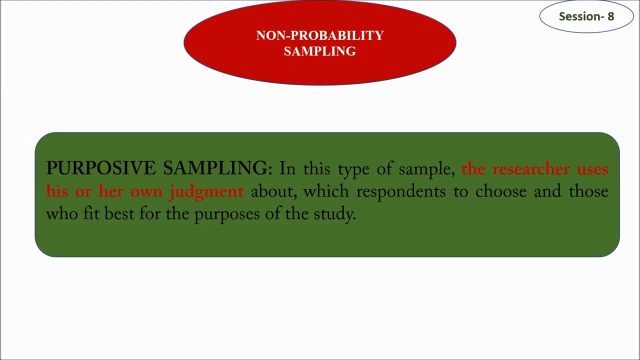 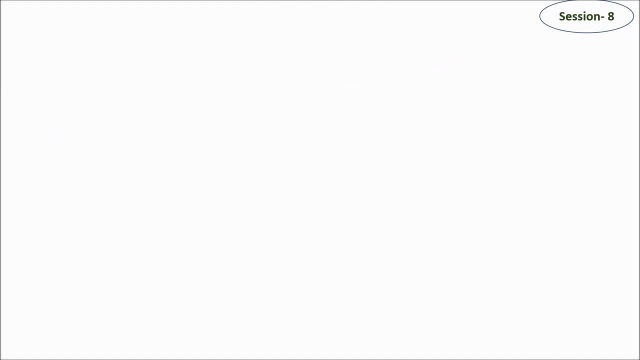 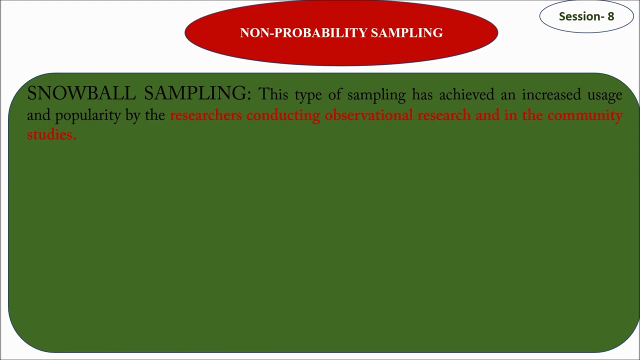 Who is the judge here? The researcher. So the researcher uses his judgment to define his purpose for the study, Using this particular sample and then snowballing. Now it's very much important. It has gained lots of importance in particular kinds of studies. 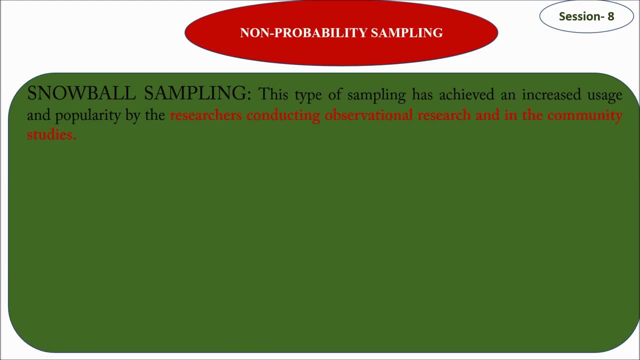 So researchers conducting observational research or community based study use snowballing. That is, snowball sampling, All right. So it is connected in stages. So first stage: we select few people who are found through interviews or through people who identify as the key informants. 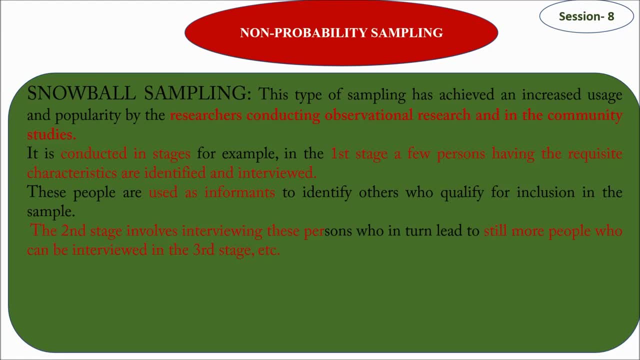 All right, And then The key informants. The second stage is involved using those people and interview with men again, And from then the third stage. So what happens? First we find one person, Then he tells us about the three more persons of the same nature. 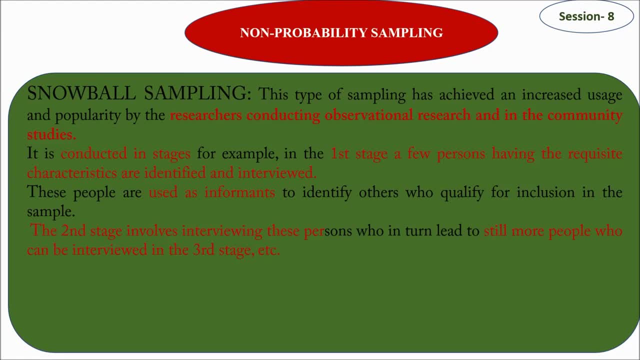 Then from these three more person on the second stage we talk to nine more people, or ten more people using them. So what is happening? It is very similar to like a snowball, like a big snowball that is being made at the base. 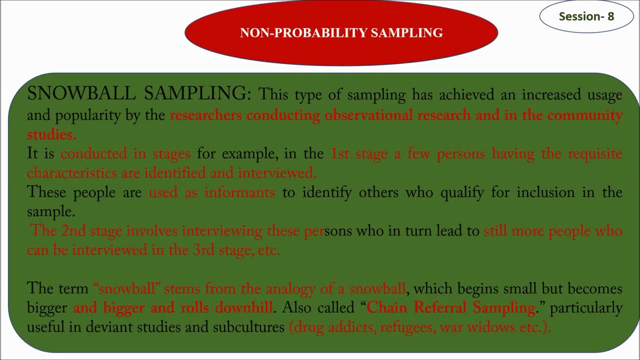 If a small snowball is rolled from the head, It is a big snowball that is being made at the top of the hilltop and gradually it picks up a snow on the move down the slope and gradually becomes a big snowball. So first you get one person in first stage, then three person in second stage, then 15%. 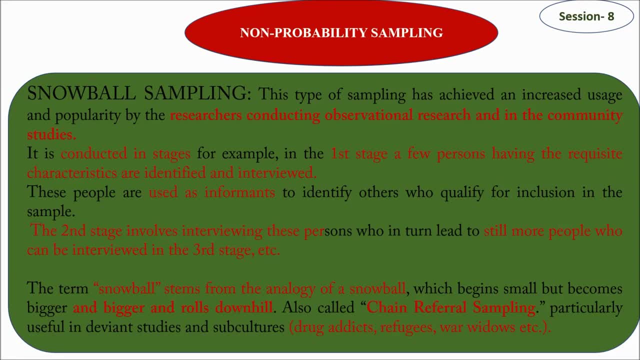 maybe All right, So largely the snowball gathers up. So this is also sometimes referred as chain referral sampling- That is another terminology for that- And this kind of sampling is importantly used in community studies and very specific studies, For example, drug addicts, refugees, war widows. 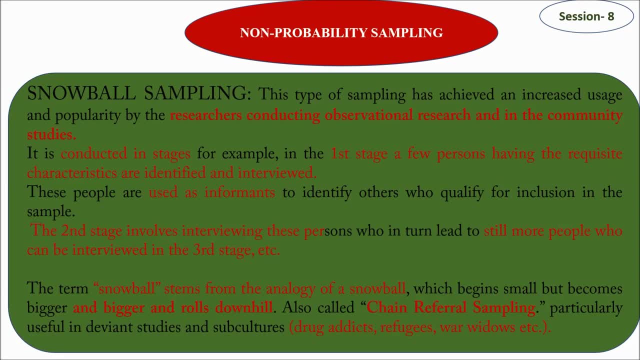 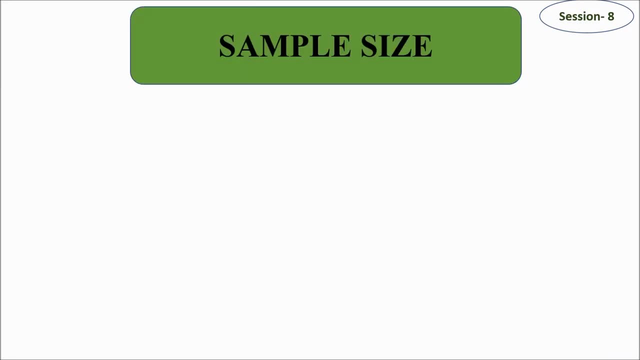 So that is another terminology for that- And this kind of sampling is important. We use in community studies and very specific studies. So such kind of sample, if you want, then snowballing, is very much helpful. All right, Now let's look at one another important point, that is, sample size. 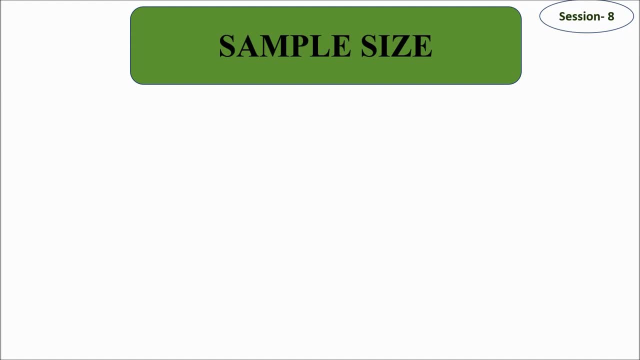 How do we select sample size and what does it mean? So sample size may be chosen based on different parameters in several different ways. So what are those parameters? first, based on experience. It means this choice of sample size through, sometimes, our own experience is important. 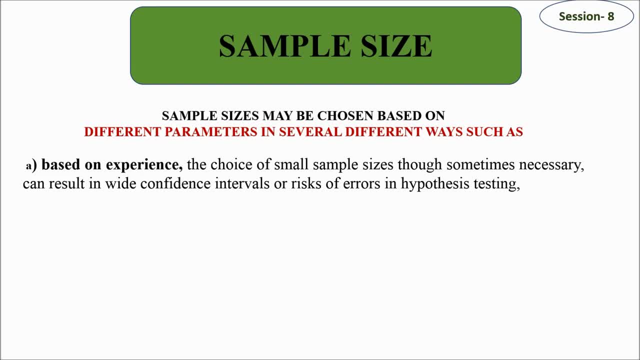 For example, we can assess the intervals or risks of errors in hypothesis testing, Then using a target variance for an estimate. Okay, So target variance for an estimate can be derived from the sample obtained. If a high precision is required, then narrow the confidence interval. 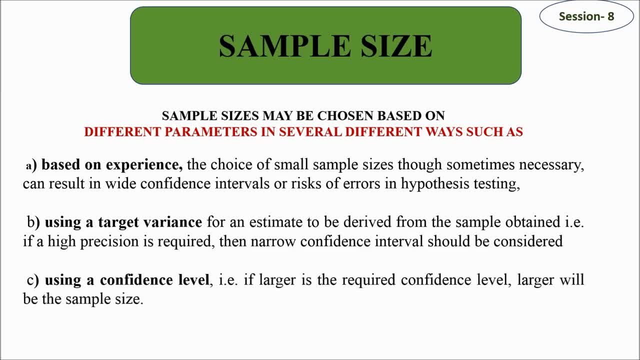 That is how it is done. And the third and the last one is the confidence level basis. So if a large, if it is a larger sample that is required At larger confidence level, then larger will be the sample size. So that is a direct correlation between sample size and confidence level. 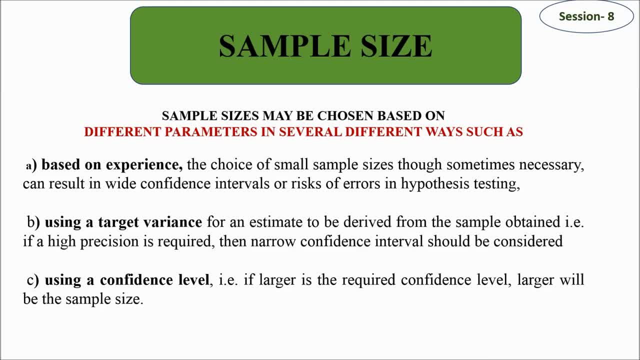 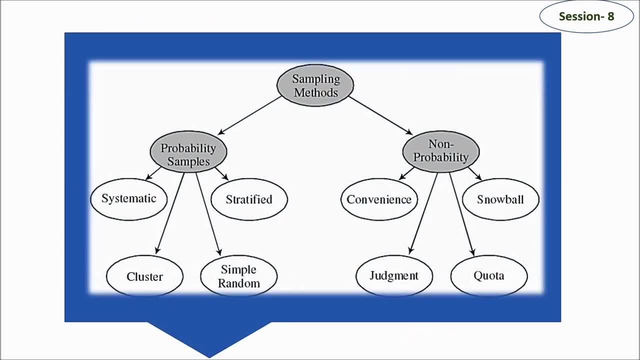 So if at a larger confidence level, larger is the sample size. That's how sample size is selected. So we can summarize the entire sampling methods into two distinct categories: probability samples and non-probability samples, under which we have several further categories. 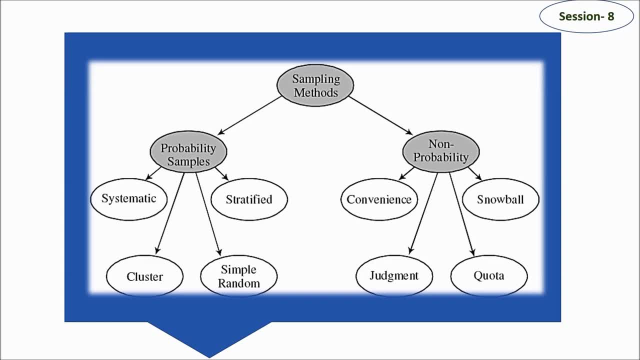 systematic, stratified cluster, simple, random, All right. So the first category is the sample size. It is the sample size that is most likely to be selected as a probability, samples where probability of being selected is there, Right, And it is claiming to be representative of the entire population or the universe. 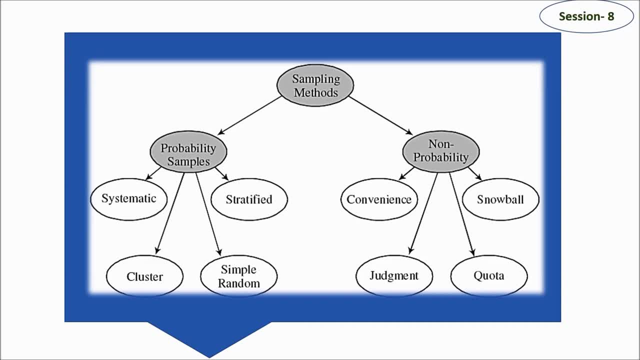 But same time, non-probability sample is based on the researchers judgment, It's based on the convenience, It's based on the specific type of sample or context of the study. So judgment and quota sampling All right. So this is the. 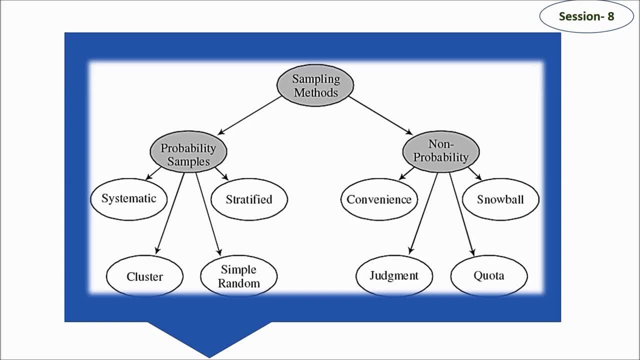 Largely The way in which the sampling method is thought to be the most possible way of Skill exempel for his research. All right, So today we completed the sampling techniques, sampling methods, its various types, its advantages and disadvantages. So please like and subscribe to our channel, the geochemist, and please press the bell. 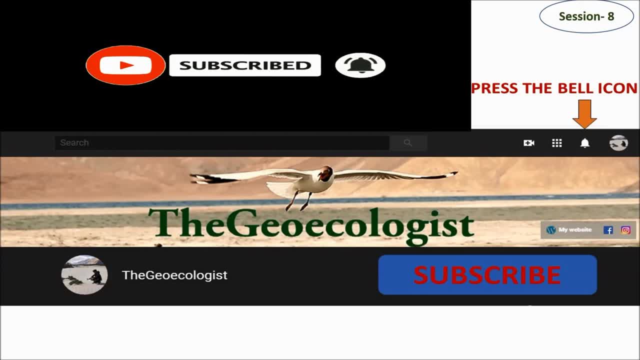 icon for the updates. Stay tuned, Stay safe. Thank you so much.